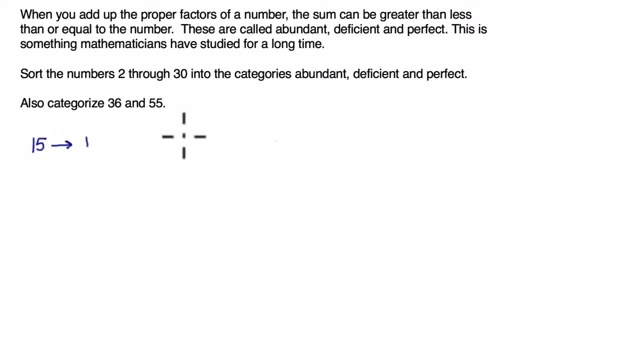 the factors of 15 are 1 times 15 and 3 times 5.. So the proper factors are all the factors of the number, except for the number itself. So in this case, for 15,, 1,, 3, and 5 would be the proper. 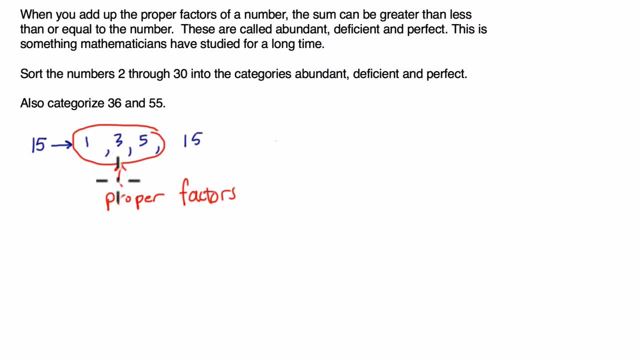 factors. And what they are saying is: if you add up these proper factors, you're going to get the proper factors, If you find the sum right. so if we do 1 plus 3 plus 5, if we add them up, 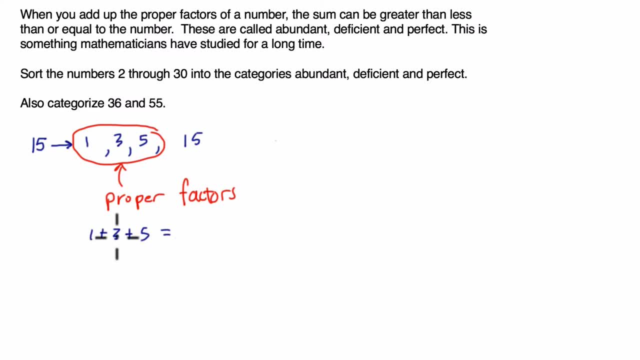 and look at that sum right, we get: 4 plus 5 is 9.. If we look at this sum and compare it to the actual number, in this case 15, we can categorize the number. If, since 9 is less than 15, the sum. 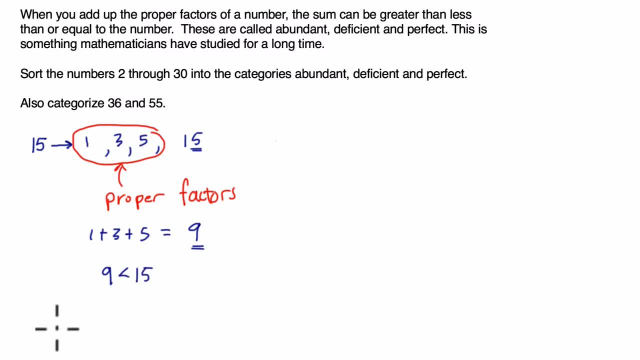 of the proper factors is less than the number, we would call this deficient. So 15 is deficient. And they're saying if you look at the proper factors of sums of different numbers, you can categorize them as deficient when the sum is less than the number. abundant when the sum is more than the number. 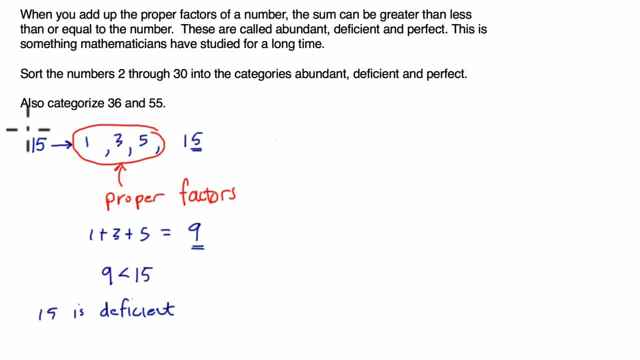 and perfect when the sum is equal to the number, And this is something that is really fun to look at and really important in a field called number theory. So they want us to look at the numbers 2 through 30 and then categorize 36 and 55. So that's a lot of numbers to factor right. So let's think. 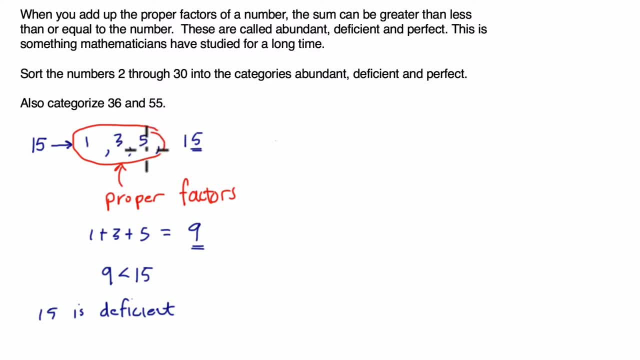 about this. When we're factoring each number, maybe we'll look for patterns. I mean, we've got 15 done already, but maybe there's a way to think about this that won't be so tedious, So let's do that. So I want to draw some circles here. These are: 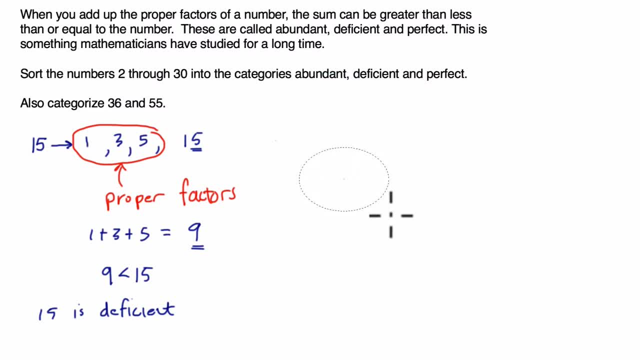 going to look like categories. So here is one circle and this will be our deficient circle. Now, there's nothing wrong with these numbers, but deficient numbers will go here, And they wanna make circles for abundant and perfect. So what will be number 2?? Well, the only factor of 2, 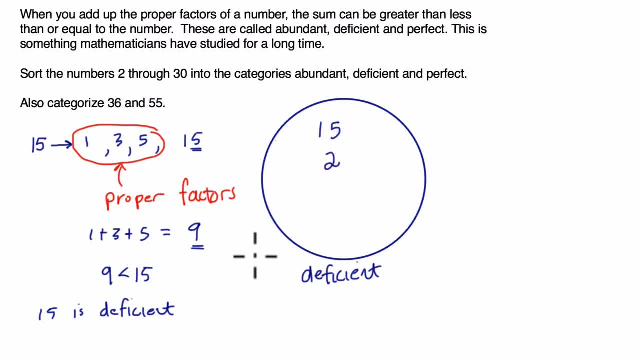 is the number 1.. And 1 is is smaller than 2, so that's deficient. The only factor of 3 is 1, and that's less than 3, so I'm starting to think: okay, I know it's. 2 and 3 are both prime, and I'm thinking all prime numbers. 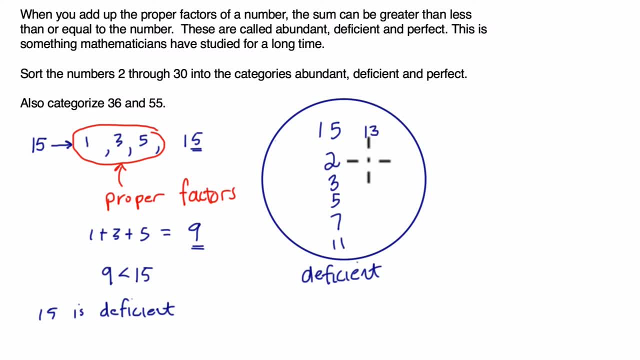 are going to be deficient, right? So I'm going to put them all in here and I'll write them down. let you think about that. for a second right: 19,, 20 is not prime, 21,, 22, 23 is prime. 24, 25 is. 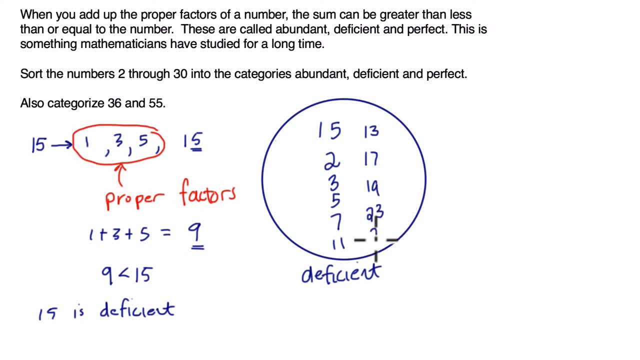 not prime. 26,, 27,, 28,, 29 is prime right. So any one of these numbers, the only factor of a prime number is going to be the number 1, and 1 is less than all the prime numbers. so all prime numbers. 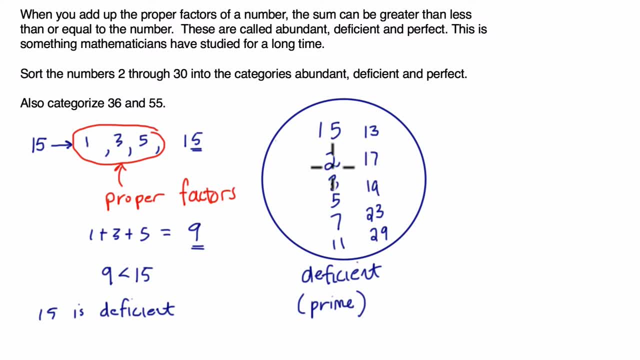 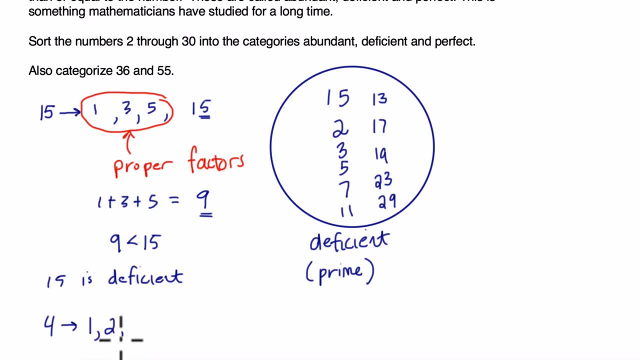 are deficient. So look at that, we got a bunch done already. So we got 2,, 3, what about 4?? The factors of 4 are 1 and 2, and 2 and 4.. So where do we put this one? Well, one little. 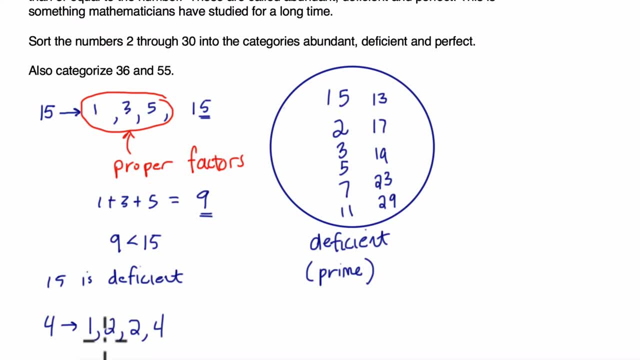 thing to think about is: what do we do here? Do we add both 2s- their proper factors, and 1, is it 2 plus 2 plus 1, or is it 1 plus 2?? In other words, do we just add the different types? 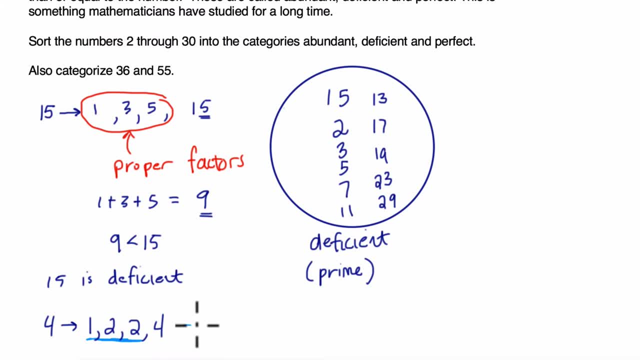 of factors, Now the convention I found. I'm not sure why this is and I'm curious to see how that changes. our answer is to only add the types of proper factors, in this case 1 plus 2, and that's. 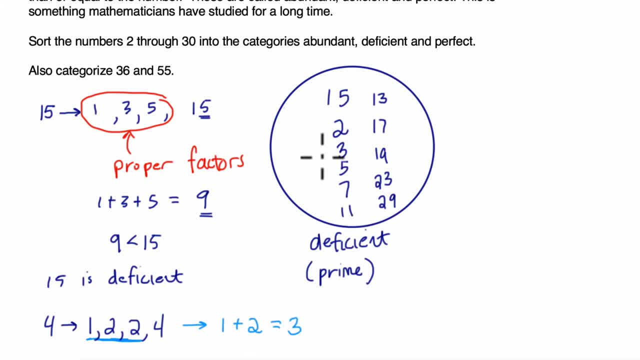 3, right. So 1 plus 2 is 3, and 3 less than 4, so we also put 4 in deficient. So when we're adding up the factors, we're going to add the types of factors and we're going to add the types of. 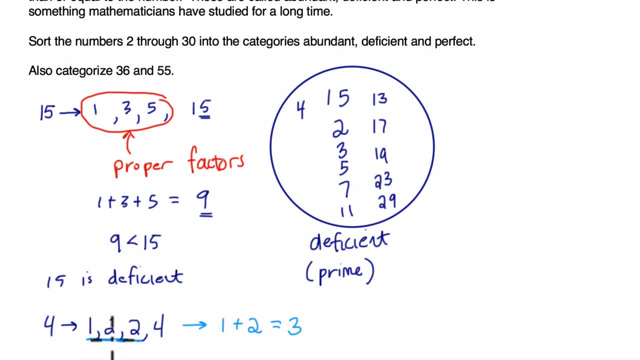 factors of a number. If you see a factor appear twice, we only need to add it once. I'm not sure why that convention exists, but it does. Now we have 5, and then we go to 6.. So 6,, 6 is awesome. 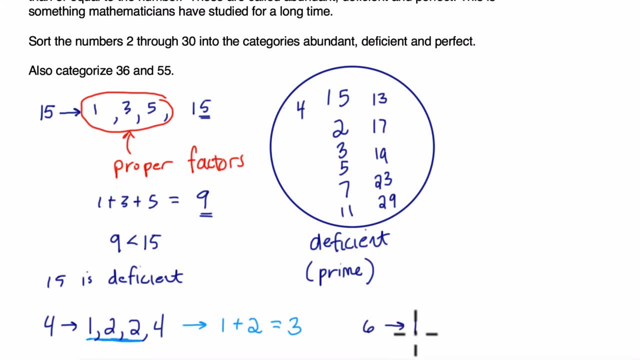 it's the first perfect number. How cool is that? What? Well, 1 times 6 is 6, and 2 times 3 is 6, and if we look at the proper factors here, right, let's say we add 1 plus 2 plus 3,. 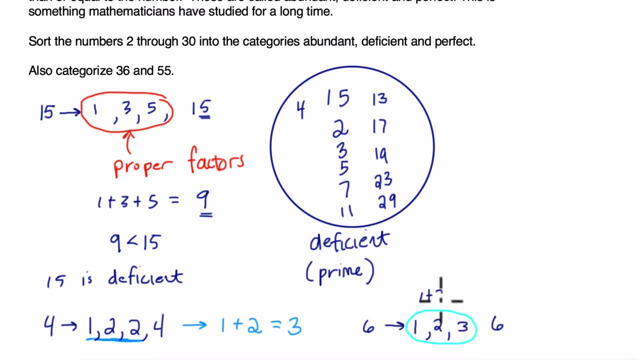 what do we get? Well, 1 plus 2 is 3, plus 3 is 6.. So what happens? right, Finally, we have a number where the sum of the factors is equal to the number itself. Now, 6 is all by itself. there, it is right, It's sitting in the 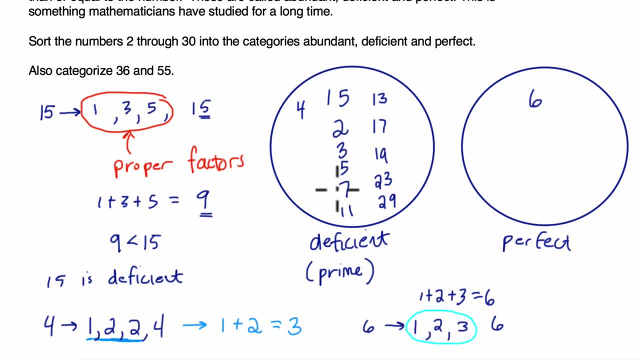 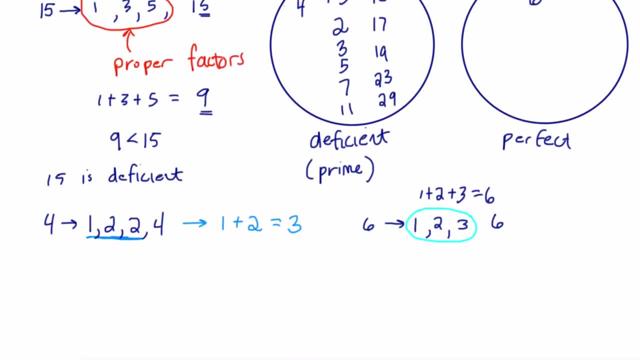 perfect circle. And now we go to 7 and have it there 8.. So now we're going to factor 8.. Give myself a little bit more room. 8 is 1 times 8, and 2 times 4.. So 1 plus 2 plus 4,. 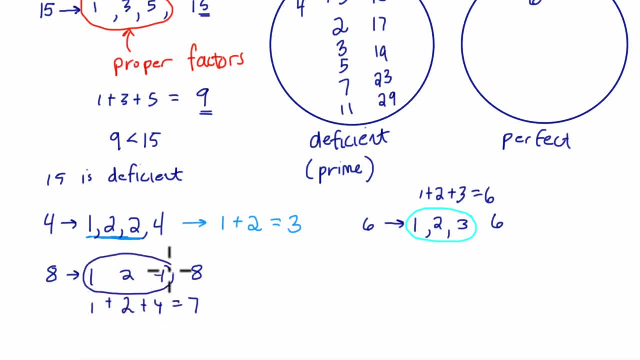 is 7.. So close to being perfect when we have those proper factors, but it's deficient. You see, this deficient category, it's like really stuffed. There's lots of stuff in here. We look at 9 next and we have the proper factors are 1 times 9, and 3 times 3.. So what are we going to? 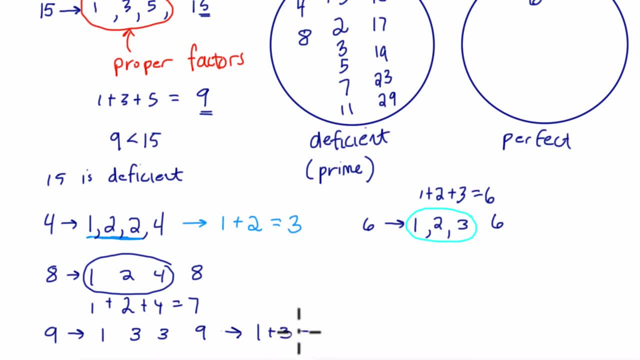 do? I'll draw an arrow here: 1 plus 3 plus 3,, which is 7, and that's less than 9, so that's also deficient. Then we go to 10, put 10 right. here We have 1,, 2 times 9, and 2 times 3,. 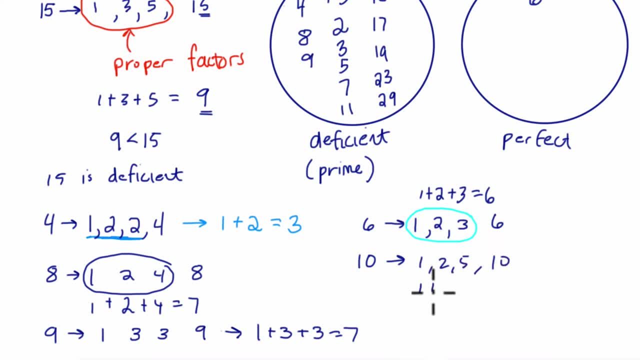 times 5, and 10.. So 1 plus 2 plus 5 is 8, and that's also deficient 11, we have 12.. What about 12?? Let's see what happens here: 1 times 12,, 2 times 6, and 3 times 4.. So if we add up, 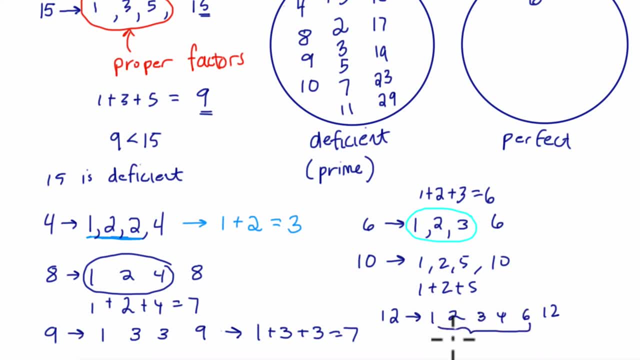 the proper factors. here we get: 1 plus 2 is 3, plus 3 is 6, plus 4 plus 6 is 10, and that's 16.. And there it is, folks, our first abundant number. So I'm going to just draw a little circle over here and write the word. 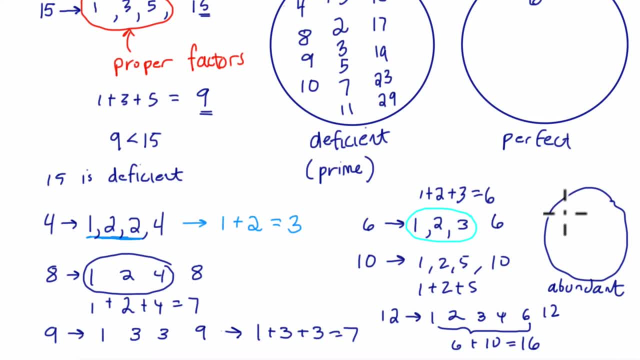 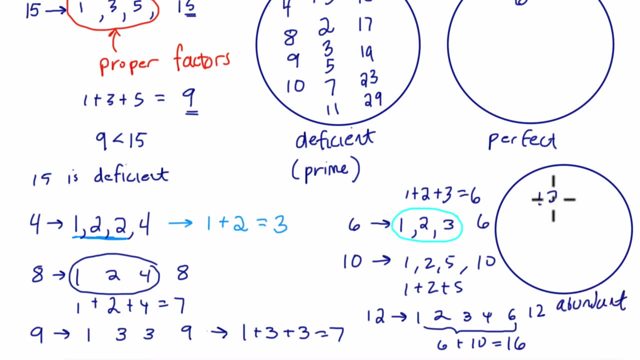 abundant and put the number. Actually, that looks terrible. Let me make a nice circle. Use my circle tool. Okay, there it is. So these are the abundant numbers and we have a 12 in there. 13 is prime. What about 14?? I'm running out of room here, so let me clear some of these. 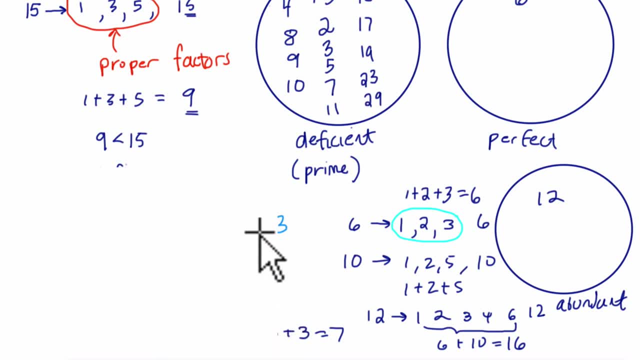 things off, We don't need all this anymore. So 14, you start factoring that number right. Oops, that was better, Okay, sorry. So 14, the factors are well 1 times 14, and 2 times 7.. So 2 plus 7 plus 1 is 9, and that's deficient. 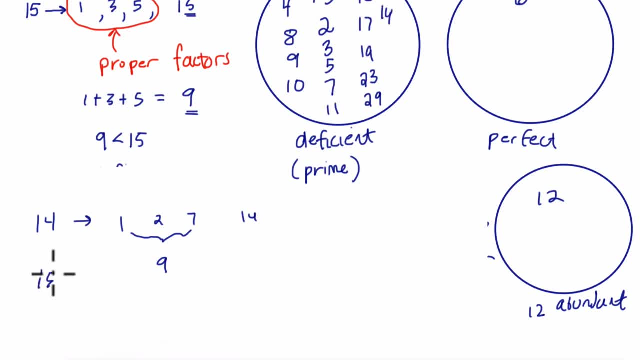 Another deficient number, 15.. Well, 15 is 1.. Let me put that down a little further: 15 equals well, the factors are 1 times 15, and 3 times 5.. 1 plus 3 plus 5 is also 9.. Isn't that cool. 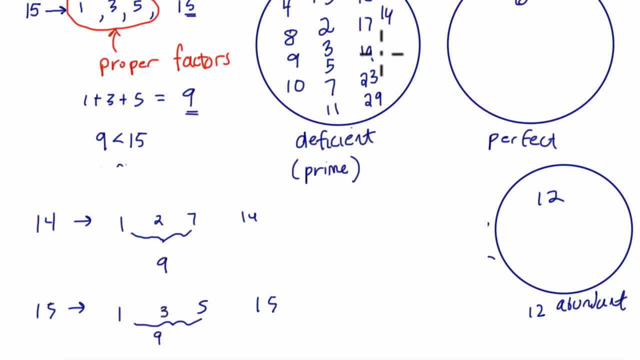 The factor sums are the same there, So that's also deficient 16.. Let's find a spot for 16.. So 16 is 1 times 16.. 2 times 8, and 4 times 4.. So if we add these up, it's going to be 1 plus 2 plus 1, 4,. 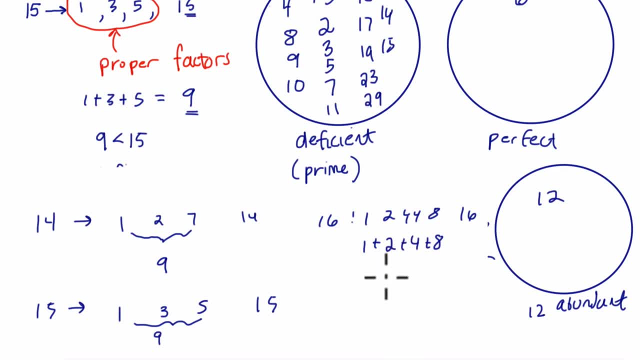 plus 8, and that's 12 plus 2 is 14, plus 1 is 15. right, so close to being perfect. so 16 is right here, 17, we have. let's do 18. well, 18 is 1 times 18. 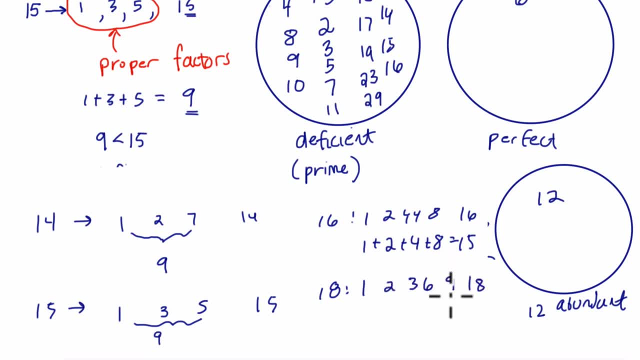 2 times 9 and 3 times 6. if we add up our proper factors here, oops, 1 plus 2 is 3, 3 plus 6 is 9. you have to add another 9, so 18 plus 3 is 21. we have our second abundant number, and i noticed that. 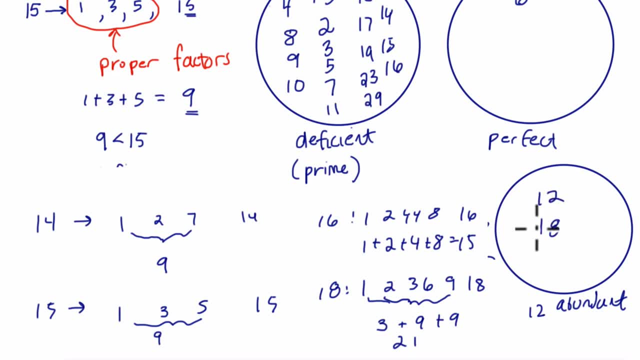 6 is perfect and the multiples of 6, 12 and 18 are abundant. so i wonder if 24 will also go here. so 19, we have right, let's go to 20. okay, clear this off. so what does 20 do? well, the factors of 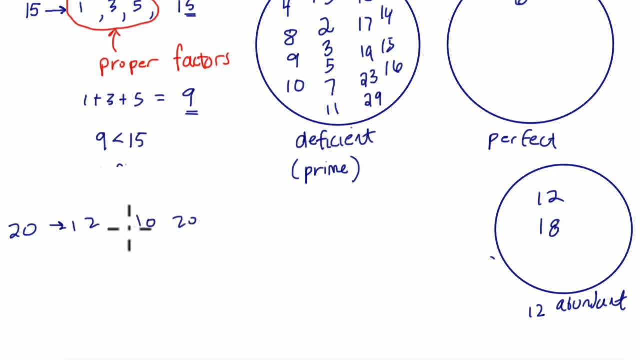 20 are 1 times 20, 2 times 10 and 4 times 5. so 10 plus 5 is 15 plus 4 is 19 plus 2 is 21, 1 plus 1 is 22.. It's an abundant number. 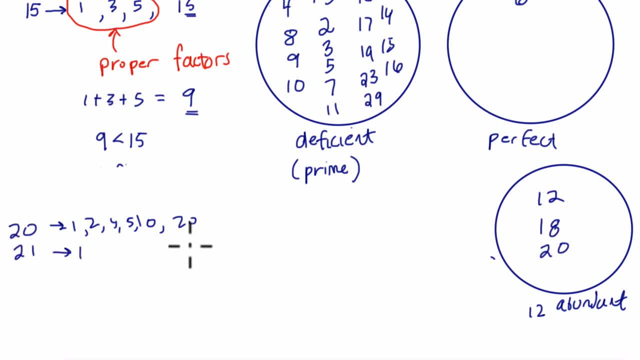 Okay, 21.. We have 1 times 21 and 3 times 7.. So 7 plus 3 plus 1 is 11, and that's deficient, Okay 22.. We have 1 times 22 and 2 times 11.. 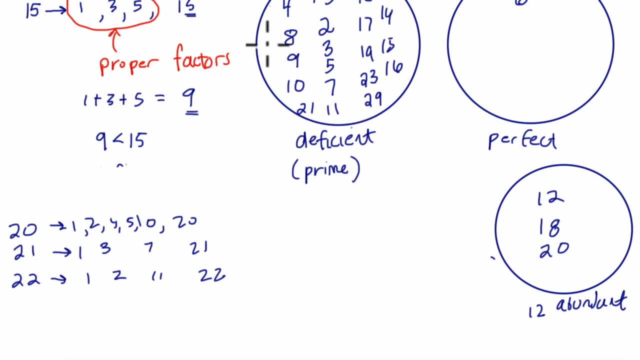 Without even adding it exactly. you know it's going to be deficient. So my deficient circle is getting stuffed here. Here. 23, we have 24.. So let's see if 24, where that's going to fall 1 times 24- is a multiple of 6, so expect it to be abundant. 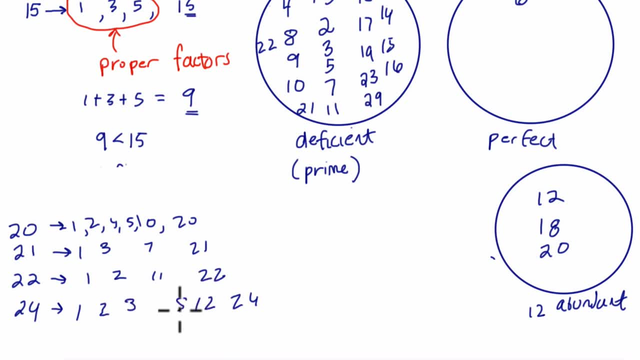 Let's see 2 times 12,, 3 times 8, and 4 times 6.. So here you can see, it's going to at least be close right. 12 plus 8 is 20, plus 10 is already 30.. 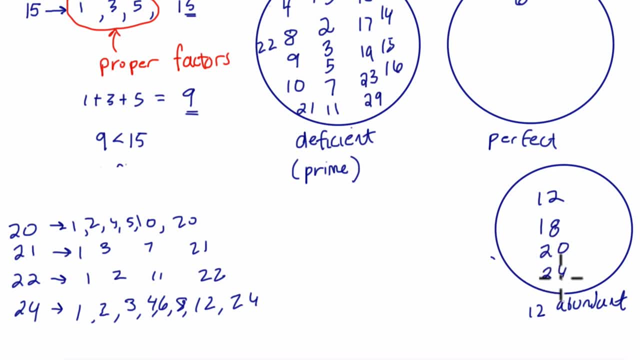 It's bigger than 24,, so it's abundant. And 25,, let's do 25.. So 25 is 1. 1 times 25, and 5 times 5.. Now let's look at 26.. So we have 1 and 26.. 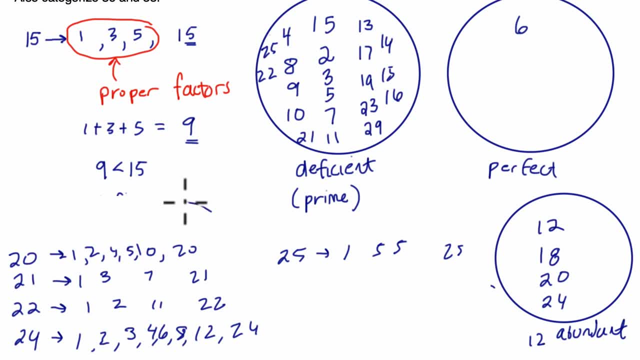 Oops. Okay, now let's look at 26.. So for 26, we have 1.. Oops, For 26, we have 1 times 26.. 2 times 13,, and I think that's it. So we have 13 plus 2 plus 1 is 16, and that's less than 26.. 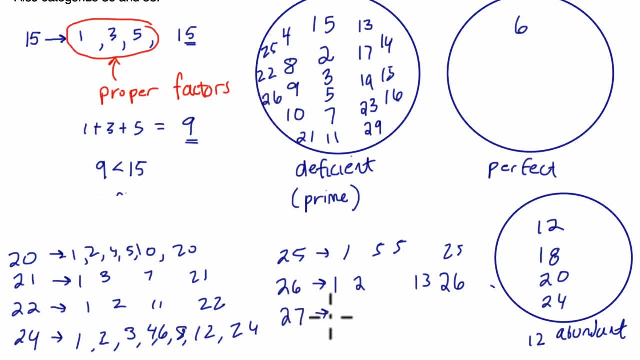 It goes here: 27.. Okay, what goes into 27?? Well, 1 times 27 is 27,, and 3 times 9 is 27.. And 9 plus 3 plus 1 is 13,, less than 27.. 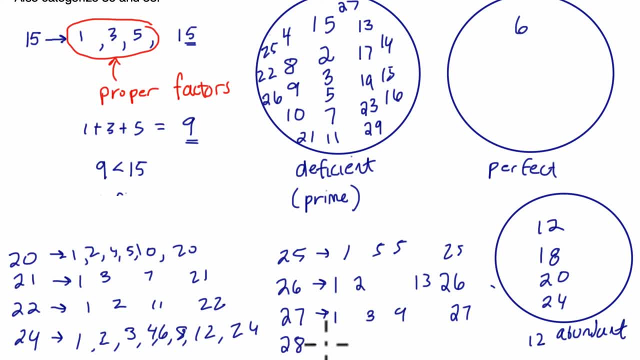 It's also deficient: 28,- we're almost there. 1 times 28.. 2 times 14.. And 4 times 7.. 14 plus 7 is 21,. plus 4 is 25,, 26,, 27,, 28.. 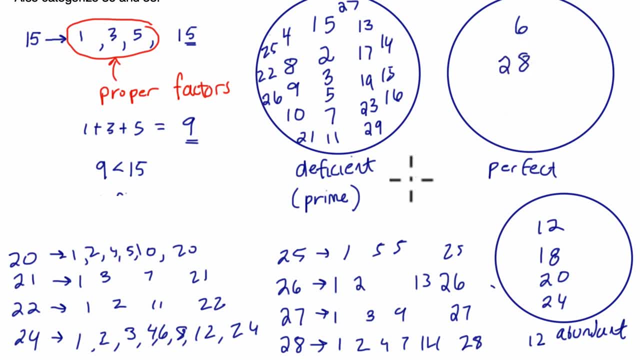 Our second perfect number. How cool is that? 29 is prime and 30,. the grand finale: 30, 1 times 30,. we have 2 times 15, and 3 times 10, and 5 times 6.. 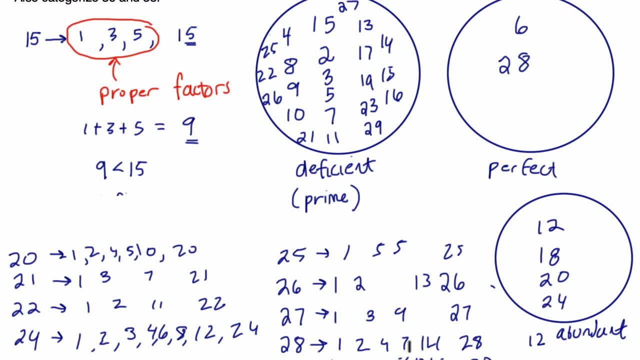 So 15 plus 10 is 25.. Plus 6 is 31.. plus 5 is 36, and then it's already bigger than 30, so it's going to be abundant. another multiple of six. so multiple of six seem to fit in this. 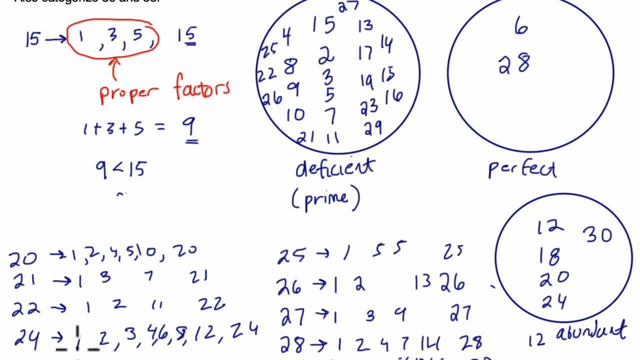 category. that's really interesting. now, two of the numbers they asked to think about are 55 and 36. let's do 55 first. 55 is odd, okay, so 1 times 55, 5 times 11, and I don't think any numbers. other numbers go into 55 I can think of. that's it so. 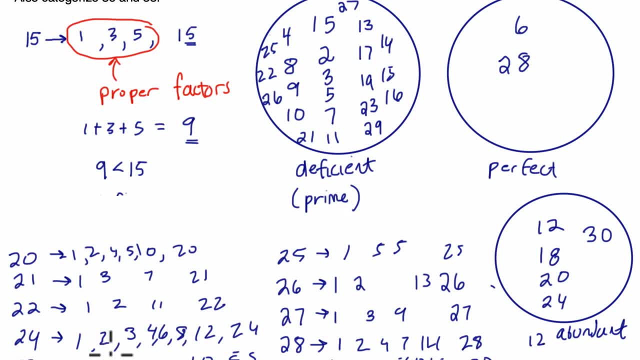 this is definitely a deficient number. we have 5 and 10 and 1 and it's 16. so the reason you see you might- I don't know if this is true, you can look into it- but it seems that odd numbers fit in deficient category and don't fit into perfect, or 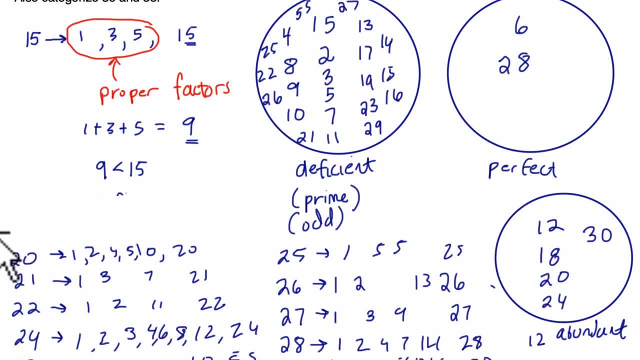 abundant. so you might look at 55 and say I think that's gonna be deficient and it seems that odd numbers fit in deficient category and don't fit into perfect, or seems to be the case. now. 36 surprised me a little bit. 36 is an abundant number. 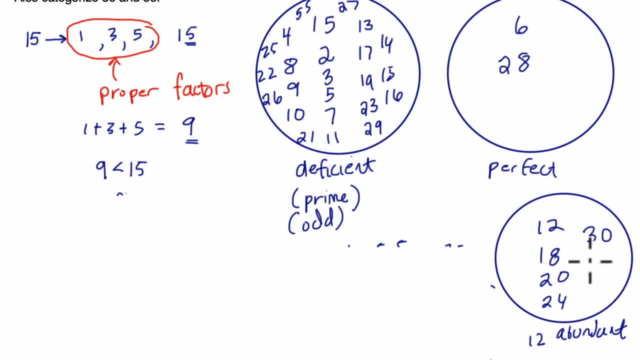 now you might not be surprised by that. could you say it's a multiple of six, but I was noticing another pattern so I guess I went 36 in gray. you look at 36, try it out. it's definitely abundant, you might. I thought it was going deficient. 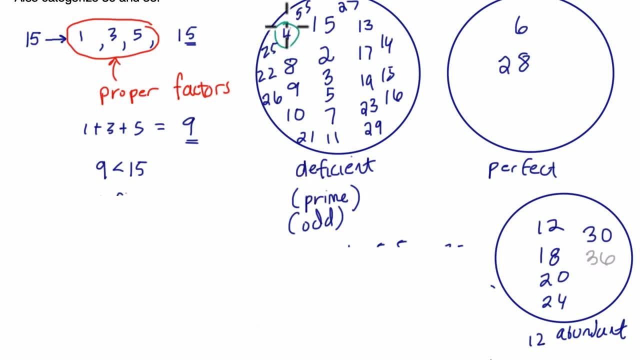 the division category because I saw something. I noticed that 4, 9, 16 and 25 are all here and those are all called square numbers. 4 is a square number because you can take 2 and multiply it by itself or square it and get 4. 9 is the next square. 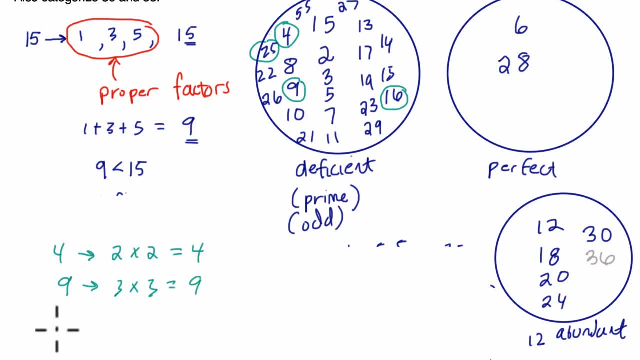 number. it's 3 times 3 and that's 9, and then 16 is 4 times 4 right and 25 is 5 times 5. so I expected 6 times 6, which is 36, to also fall in this category. 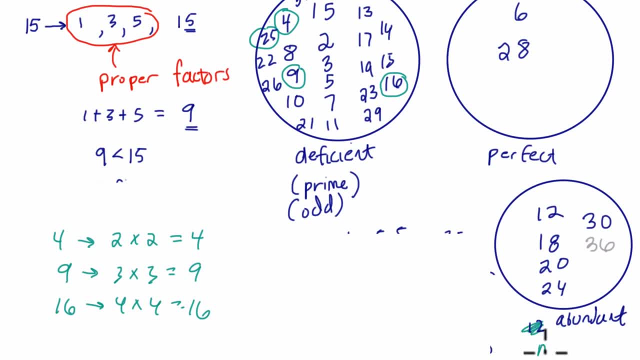 but it seems to me that multiples of 6 fall in the abundant category, so you might expect that to go here. I thought square numbers fall in deficient category. I, I'm, I'm thinking this prime number is squared. say prime squared, go here. and what am i talking about? prime squared? well, 2 is prime, the only. 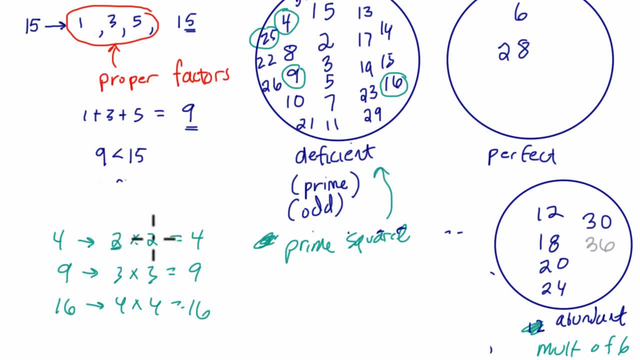 factor of 2 is 1. if you take a prime number and multiply it by itself, I think it's always gonna fall into deficient category because it makes a number with a really small amount of proper factors all right. well, I hope this helped. you can see there's lots of patterns to explore here. a really curious: what the 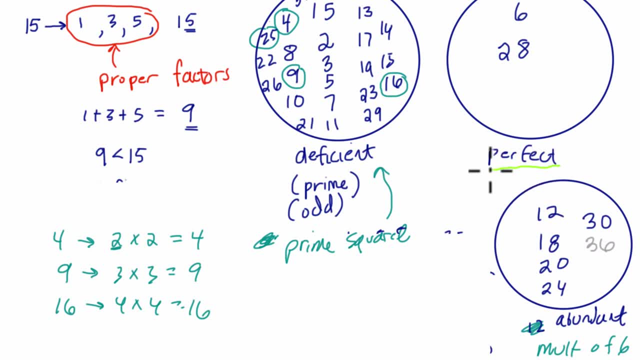 the perfect numbers, and I hope you are too. There's certainly a lot more to think about there. There's some famous theorems around it. Deficient numbers are fun to discover and so are abundant, And the point is, there are.